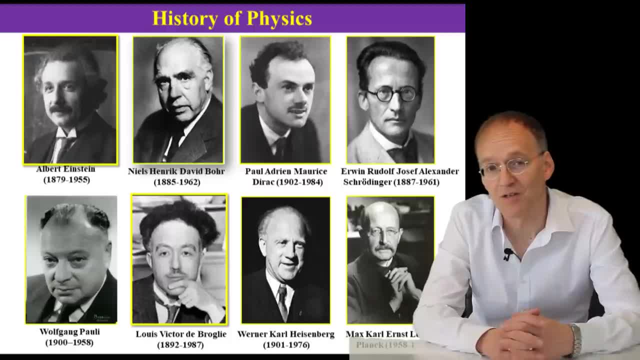 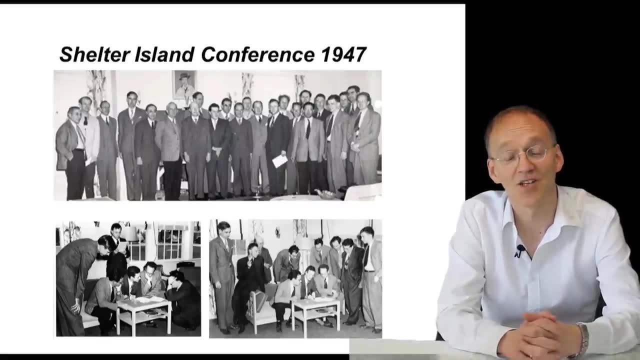 facts. I learned these facts from a Spanish scholar I will name later. and well, by the way, these facts are undisputed. You can check every single argument in the links below here. The birth of quantum electrodynamics, so to speak, was a conference in Shelter Island. 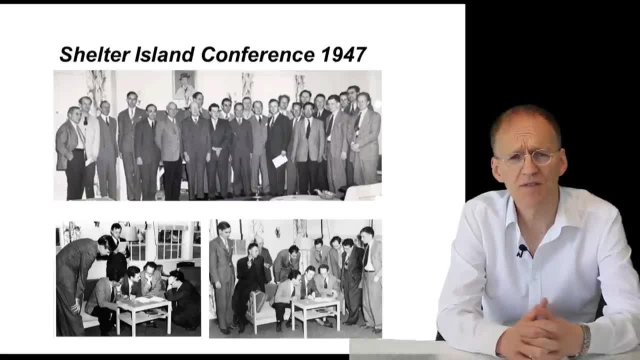 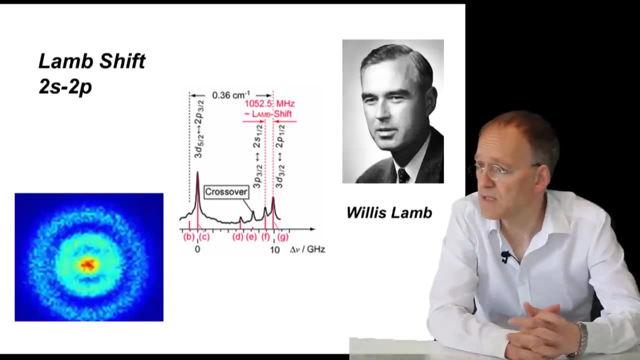 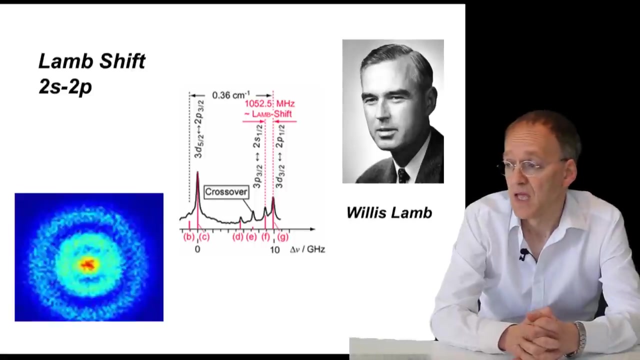 in 1947 and it was the first important post-war gathering of physicists and interestingly, no one of the early generation participated. The radar technician, William Lamp, Willis Lamp sorry, reported about previously unknown shift in the energy levels of the hydrogen atom amounting to approximately 1050 megahertz. that's the 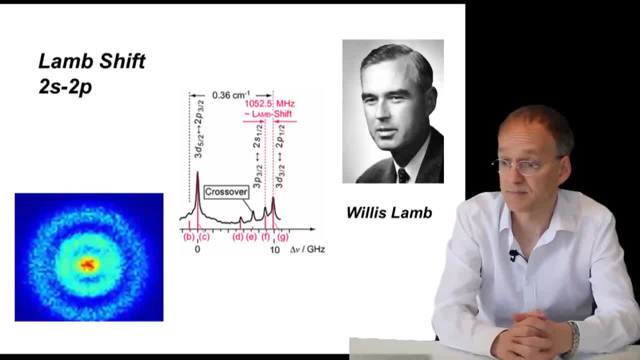 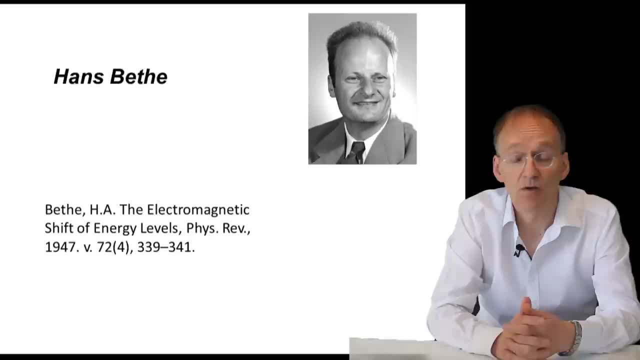 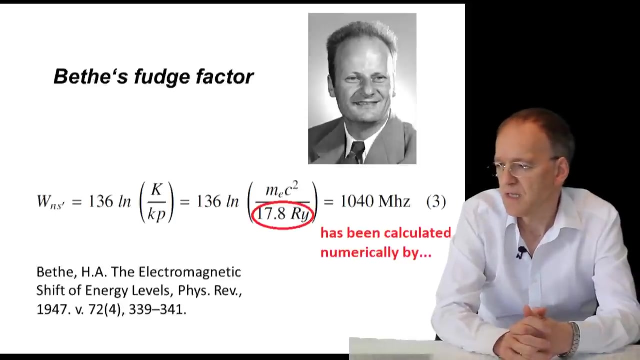 frequency, you need to lift the electron to the higher energy level. And then Hans Petty, the former head of the theoretical division of the Manhattan Project, calculated this number by using electrodynamics. This stirred the community, even though it was an approximate calculation. So if you look up the original paper, you see that in this equation Petty introduced an arbitrary number as a cutoff in the 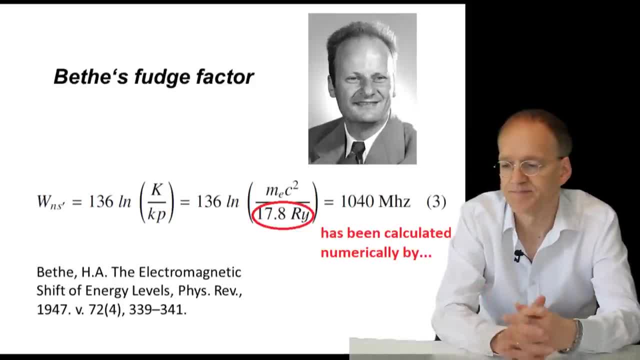 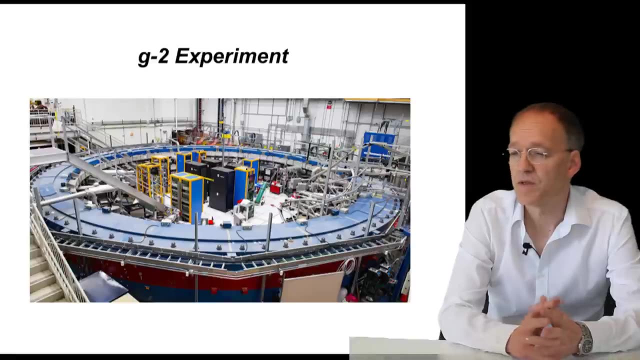 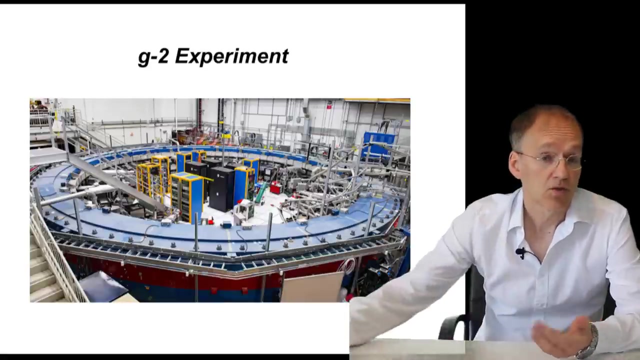 integral, and you might even call this a fudge factor. But wait a second. there is a more elaborate theory and there are more tests, one particularly impressive one with the magnetic moment of the electron. This g-factor can be measured with an incredible precision in this g-2 experiment. and well, you surely have. 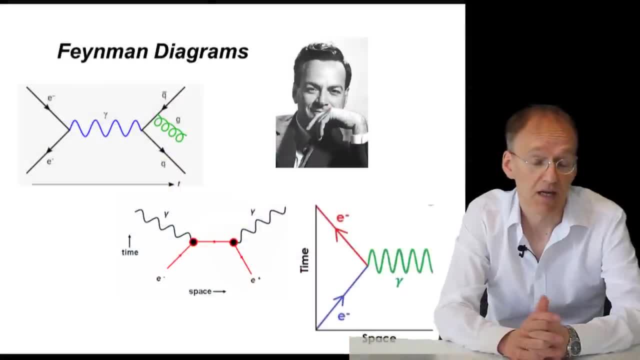 heard about Richard Feynman and the graphs named after him. These are a really nice idea about what might be going on on the microscopic level, with light quanta creating electron-positron pairs and these pairs annihilating to light again. So the idea was that the first graph contributes a tiny. 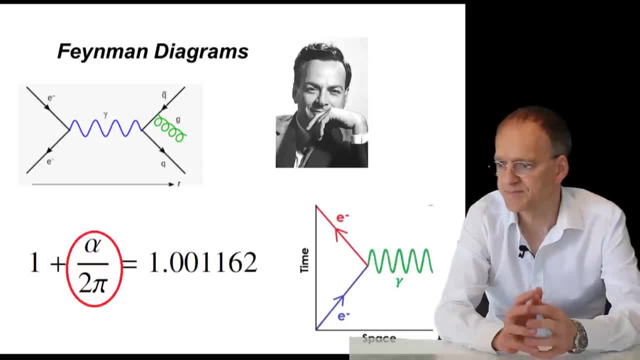 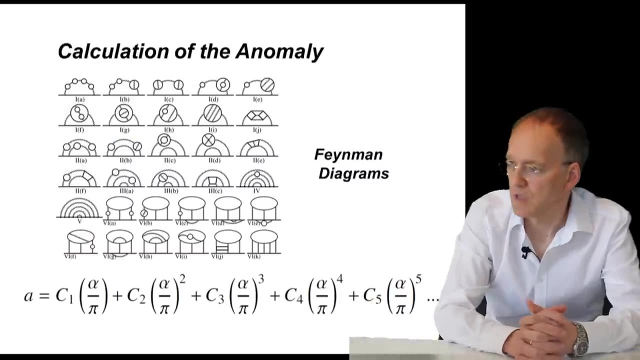 correction to this g-factor and this tantalizingly resembled the experimental measurement at the time. So Feynman made up a theory with all these kinds of processes involved and that should reproduce this g-factor. Yet in detail. it was a little bit complicated because for every process you had to calculate numerically a. 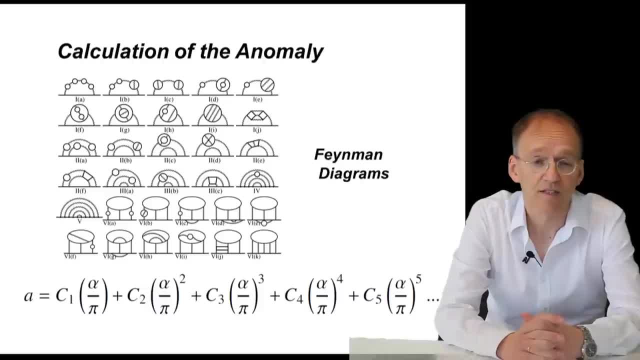 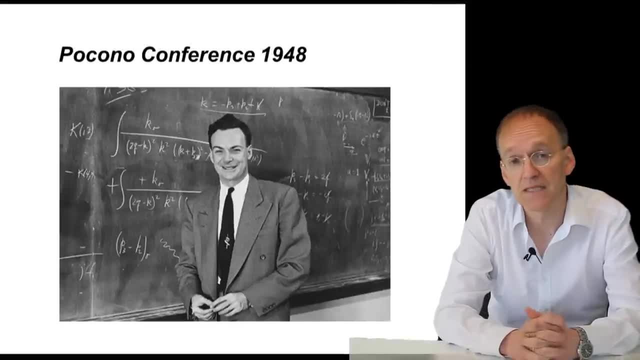 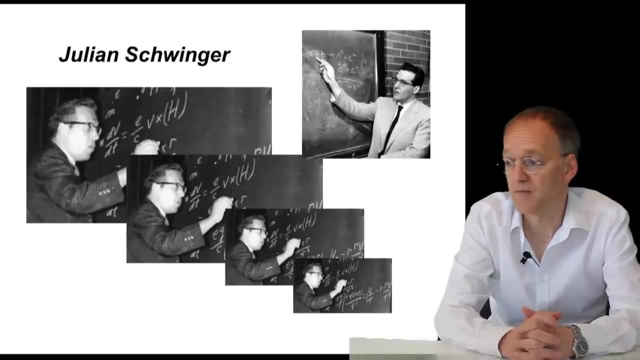 corresponding factor. Lacking any precise formulation, however, it was not surprising that Feynman, at the follow-up conference in Pocono in 1948, could not convince anyone of the mathematical correctness of his theory. So maybe it wasn't bad that the talented young mathematician came up with a very 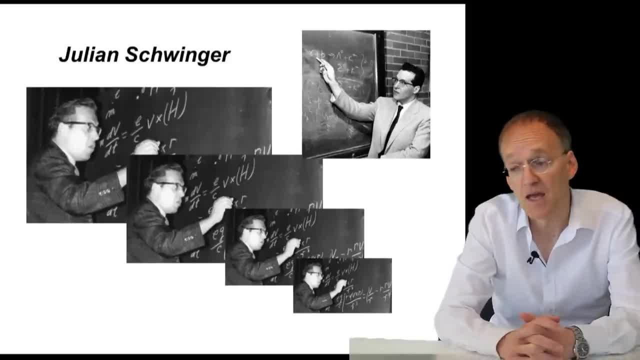 technical version of what was called quantum electrodynamics. However, his presentation lasted for six hours- no joke- in which almost everyone left or fell asleep, So this wasn't very convincing either. By the way, if you have read Feynman and Schwinger, they admitted that they did not understand. 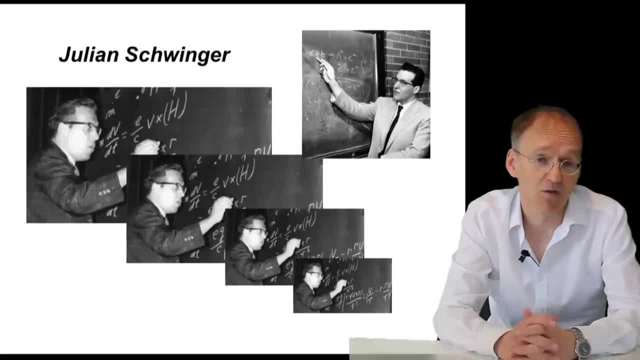 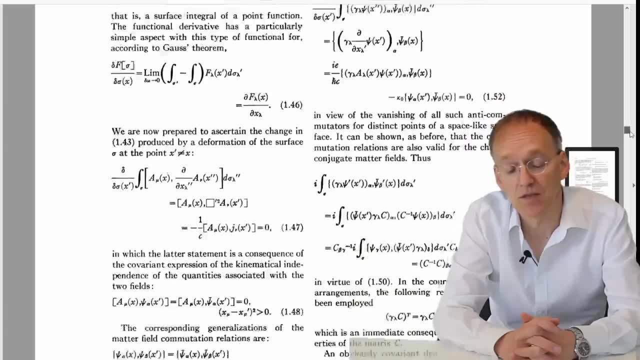 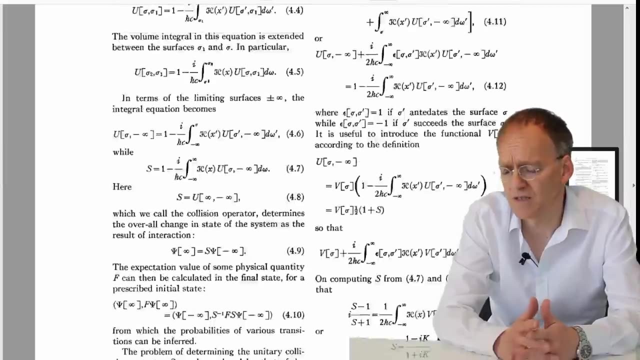 each other's theory. Nevertheless, they were convinced that they were on the right track. So you might hope to get enlightened by Julian Schwinger's papers in 1948 and 1949. However, they contain 469 formulas and it's a little bit hard. 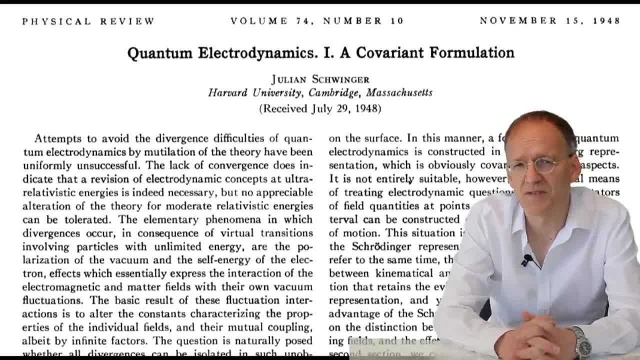 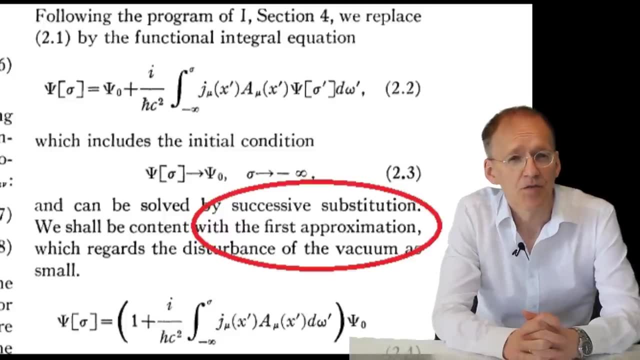 to believe that this is a precise description of the simplest particle in the universe, Especially because Schwinger admits in the first paragraph that it's just an approximation. But there was a third theory of the Japanese physicist Shinichiro Tomonaga. Unfortunately, it was seemingly incompatible with both. 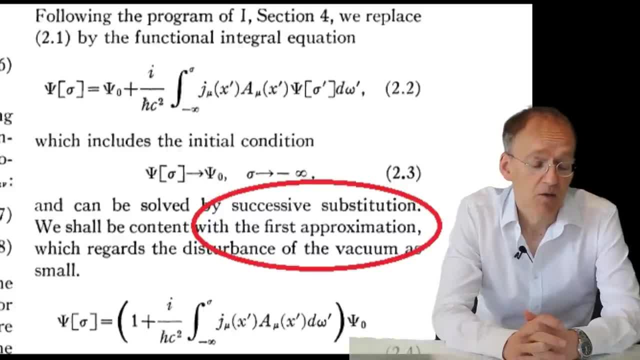 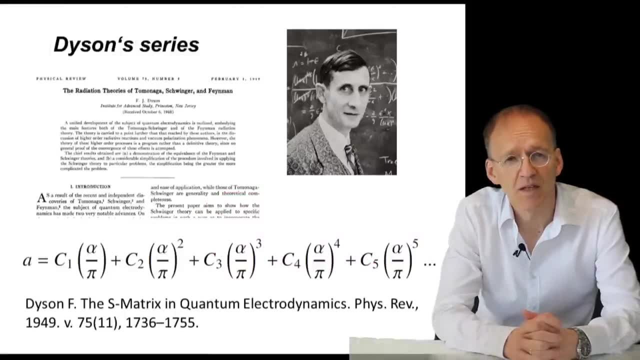 Schwinger's and Feynman's version. So eventually, to everyone's relief, the English mathematician Freeman Dyson formalized the ideas and published a landmark paper claiming that the theories of Tomonaga, Schwinger and Feynman were all the same. Dyson would come out with a bombshell revelation later, but his 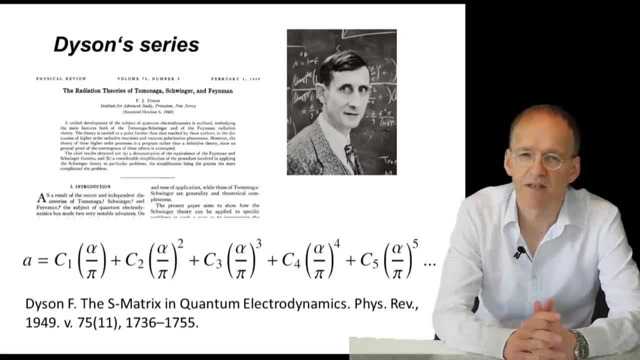 1950 paper caused excitement in the entire physics community, Although Dirac, Oppenheimer and Fermi remained quite dissatisfied with the result. Feynman's diagrams should become the popular lens of investigation. As a result, the paper language theoretical physicists use to this day. And now came the triumph of the. 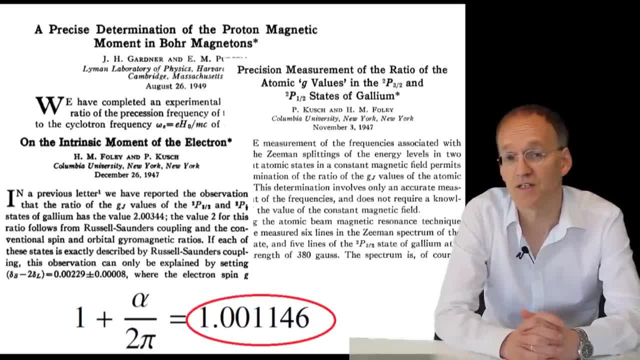 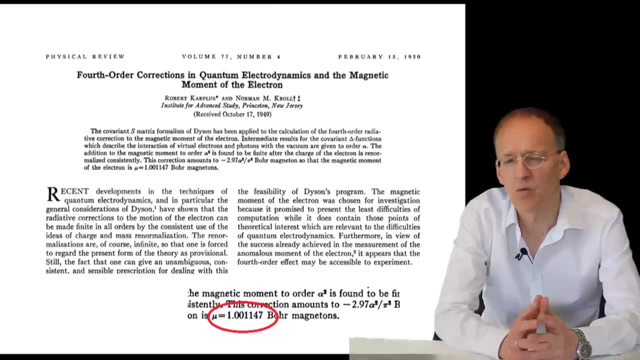 theory. The experimentalists Purcell and Gardner in 1949 had determined a new value for the g-factor, and the theoreticians had improved their calculations by correcting for another seven Feynman diagrams. Actually it's quite a complicated thing to do, but who else could do it correctly if not the 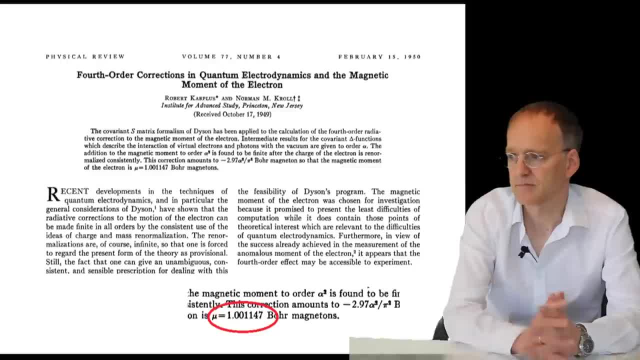 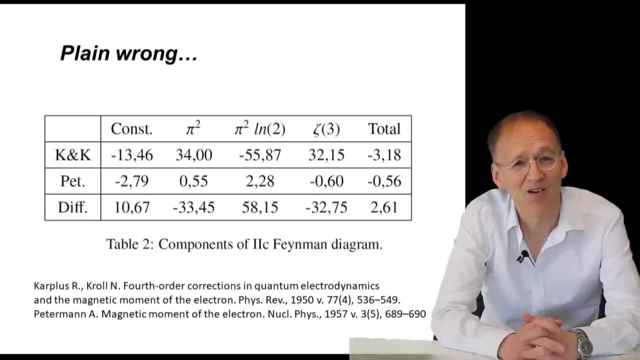 assistance of Richard Feynman, Kaples and Kroll, And say with this: it is an amazing agreement- almost in the sixth decimal place, except, well, except it was wrong. Not only also the experimental value that had matched so miraculously. 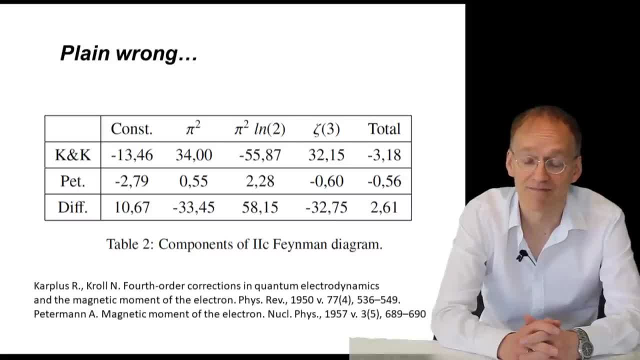 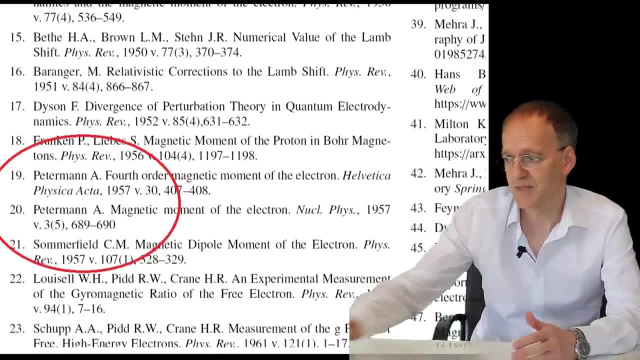 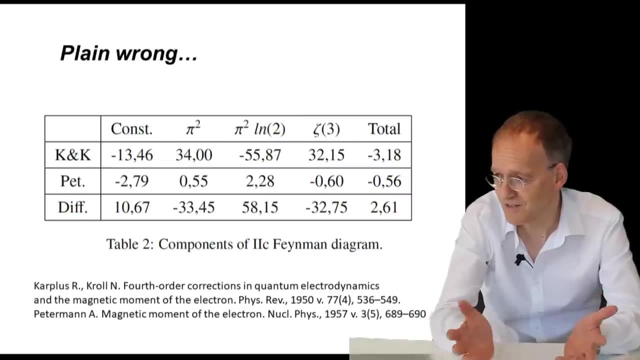 the prediction turned out to be wrong. This error was revealed seven years later in another paper by Peterman and Sommerfeld. and look at this. I mean, every single value is different here. and of course, again, Peterman and Sommerfeld were convinced that their result was correct, and maybe 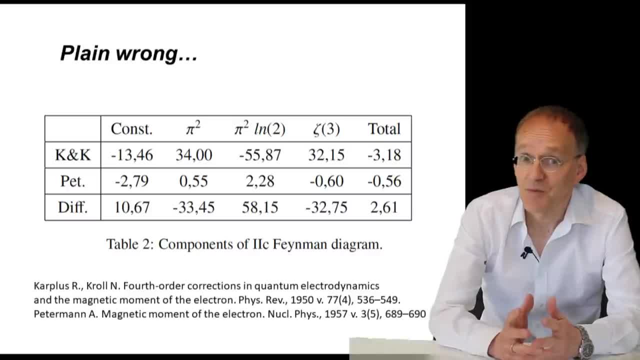 it helped a little bit that the experimental value of the time published, coincidentally one year earlier, was in agreement with the result. Well, let's pause here for a moment and keep track. Until then, no theoretical result has withstood later scrutiny. How could such negligence occur? 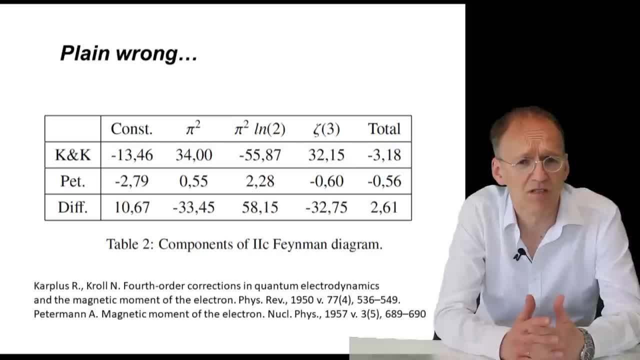 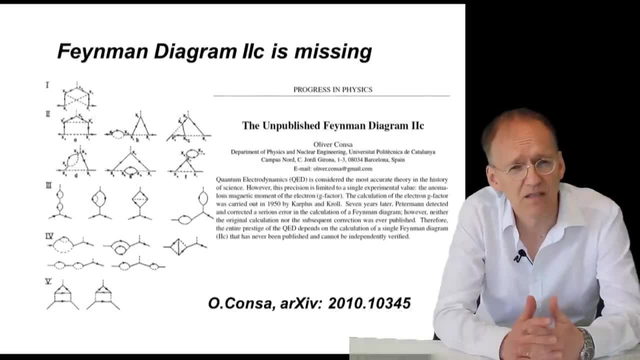 The calculations, after all, had been reviewed and published right, Well, not even published. A major ingredient of what is called the most precise theory of modern physics, the Feynman graph 2C, remained somewhere in the notes of people who died 10 years ago. Can you believe that? 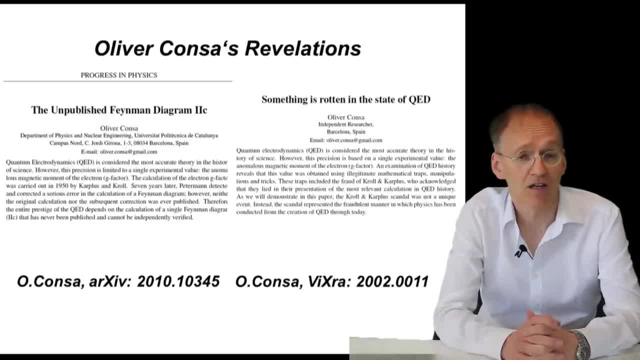 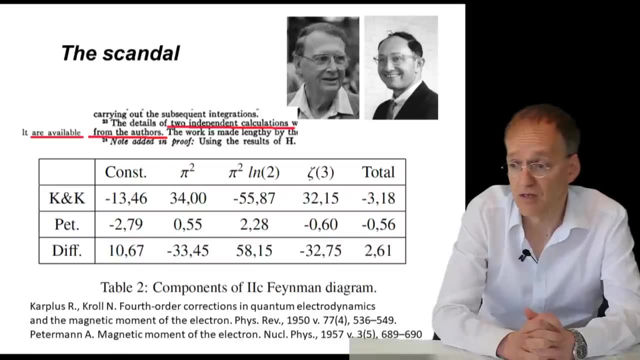 Well, if not, just check this excellent work by Oliver Konzer, a scholar from Barcelona, and I can only recommend to read his two papers. It's incredible stuff. Konzer also showed that Corpus and Kroll deliberately lied about how the calculations 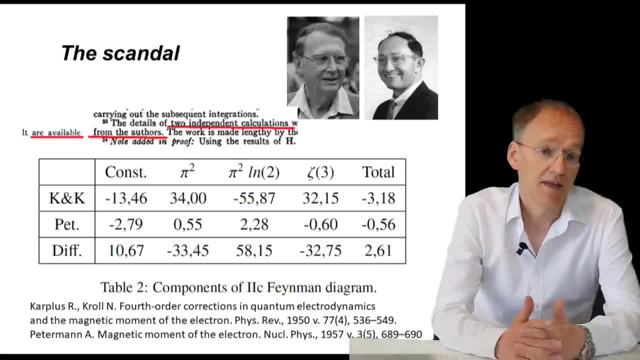 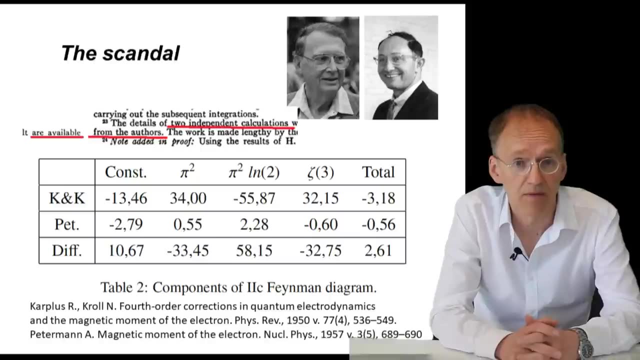 had been done, and this is a major scandal. Until then, so-called theoretical predictions had been adjusted three times to experimental values, and those again would turn out to be erroneous. So the theory is not even unpublished and wrong. Well, it is not even wrong. 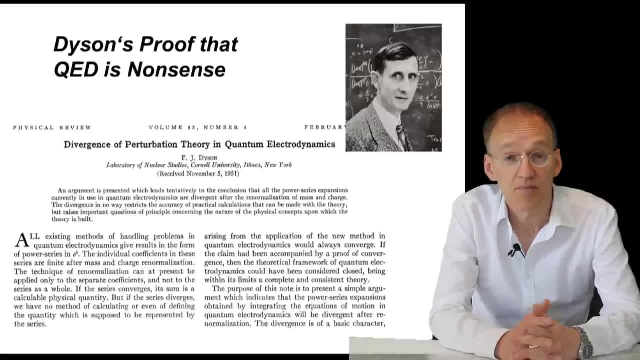 And here Freeman Dyson again comes in. He proved in 1952 that the series on which everything is based is mathematical hogwash because it does not converge. There is no point in using a series that does not converge because it may yield any nonsense. It destroys the very 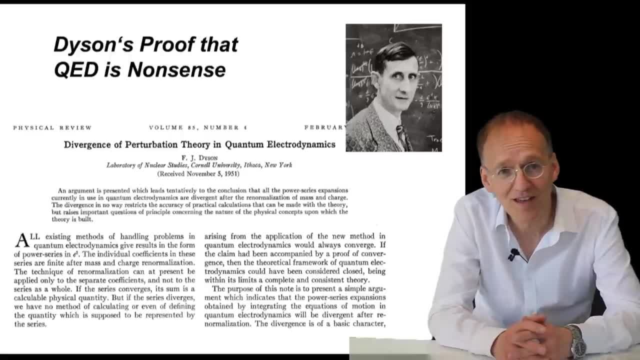 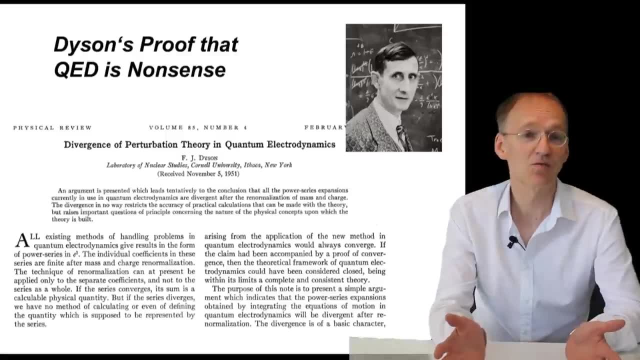 basis of what is called perturbation theory in physics. Used, say, in aeronautical engineering, it would send your aircraft crash and burn, so you would never use it. But in the fantasy land of theoretical physics you get a Nobel Prize for it. 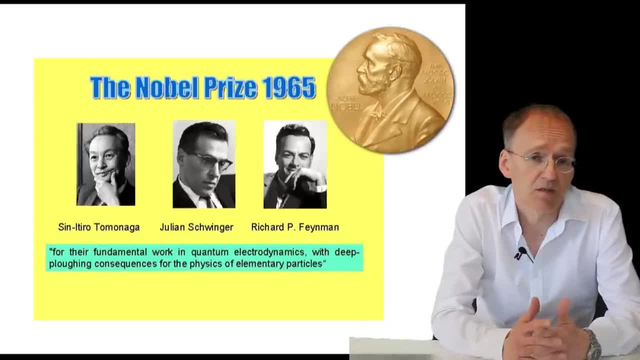 Dyson's proof was a bombshell, but it seems that the explosion took place in a vacuum, not sending the slightest shockwaves to anyone. Dyson probably was embarrassed. He moved back to England and stopped working in the field and was absent at the Nobel ceremony, Tellingly. 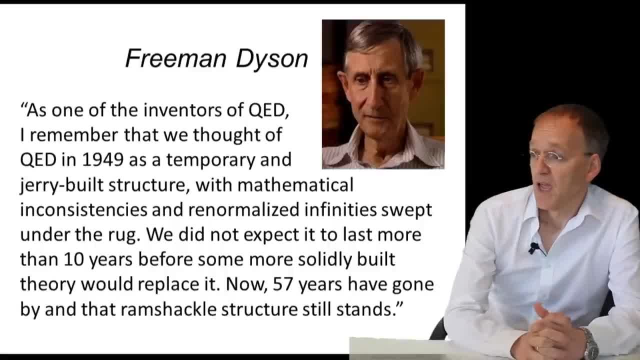 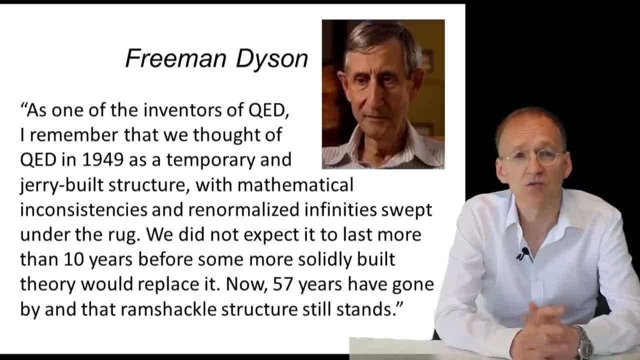 in 2006,. he confessed in a letter As one of the inventors of QED. I remember that we thought of QED in 1949 as a temporary injunction. It was a temporary injunction, but it was a temporary injunction. 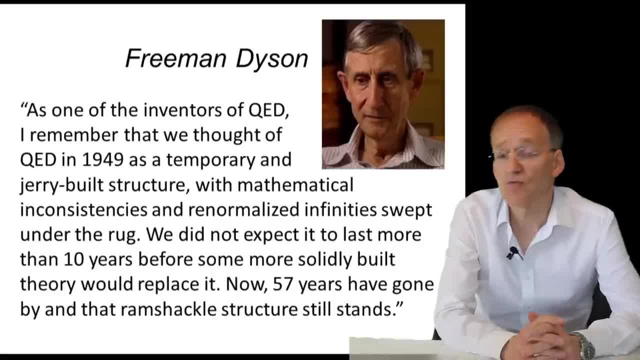 It was a theory-built structure with mathematical inconsistencies and renormalized infinities swept under the rug. We did not expect to last it more than 10 years before some more solidly built theory would replace it. Now, 57 years have gone by and the ramshackle structure still stands. 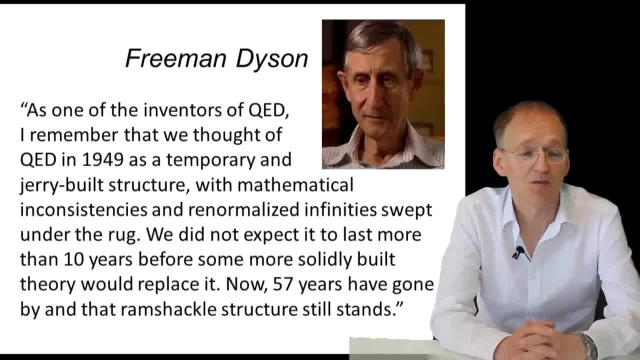 Yes, it still stands in a sociological manner, because physicists continue to parrot what a wonderfully tested theory it is. Let's open an important sideline here. You never understand physics from this tiny focus on the present. It is imperative to have a look at the history of how things evolved. In this case, it is the merit. 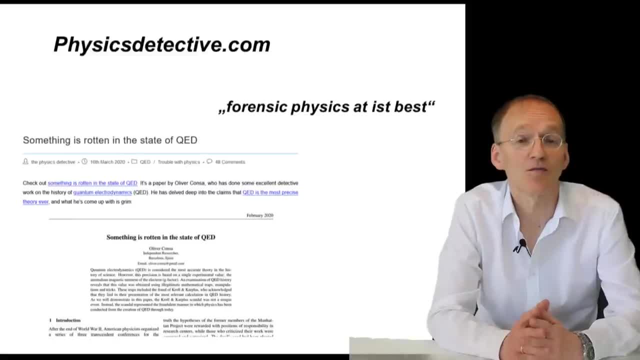 of Oliver Konzer, who did this piece of forensic physics at its best, as my friend John Duffett calls it, And if anyone, Konzer should get a Nobel for demonstrating that this allegedly best theory of modern physics is a mere illusion. 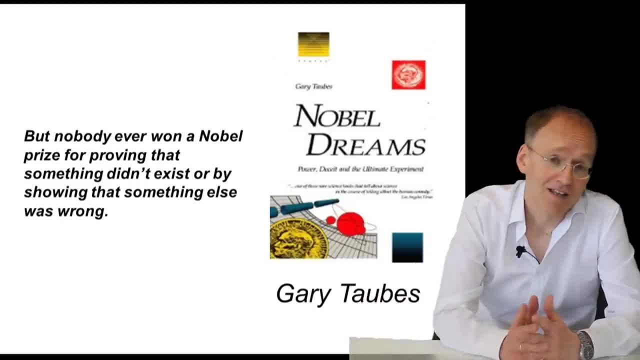 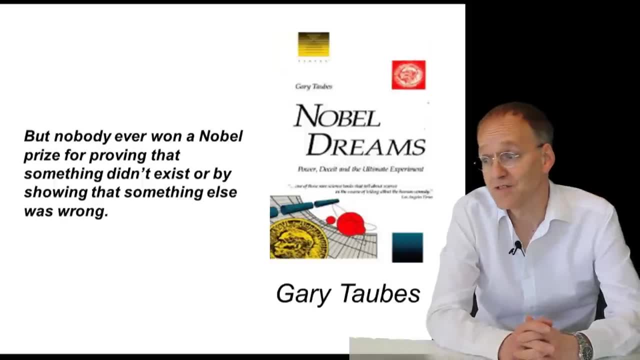 Unfortunately, it's unlikely to happen, because one of the axioms of the Royal Academy is that nobody ever won a Nobel Prize for showing that something didn't exist or for showing that something else was wrong. It is essential to look at history because, as the collective deception 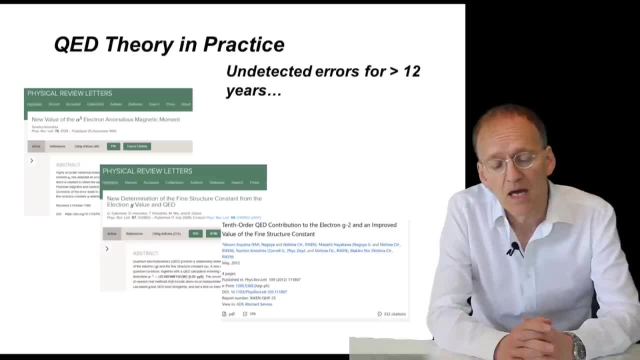 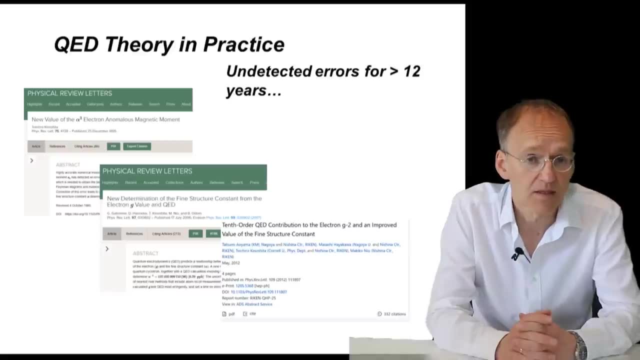 spreads, it becomes less visible. I had noted that the later papers by Kinoshita in 1995 and 2006 contradicted each other and that nobody had detected the error for 12 years. but I admit that earlier I also had participated in that choir parroting that QED was a precisely tested theory. 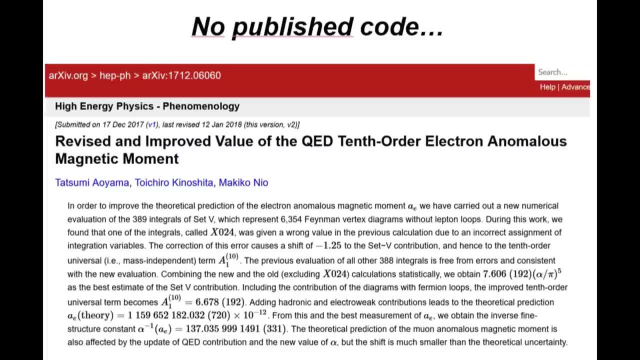 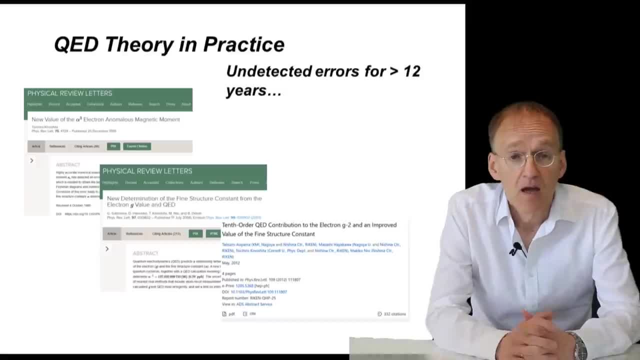 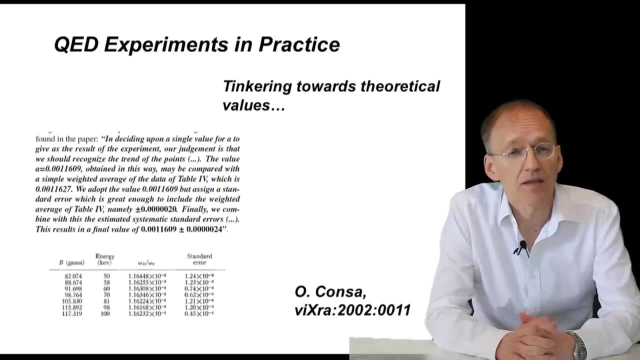 And keep in mind that practically nobody can check the correctness of such papers based on highly complicated and unpublished computer code. There were other scandals that followed, as Konzer pointed out, And sadly not only theoreticians tinkered with their calculations, also experimentalists. 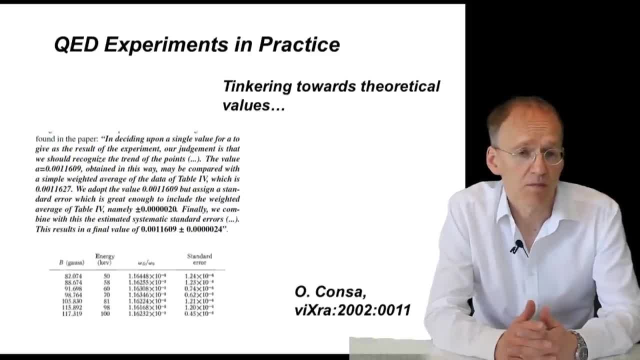 seemed to have fudged their data, because how else to explain that in 1961 they again measured a value that precisely matched the theoretical predictions that turned out wrong afterwards? Although this could be a deliberate fraud, I don't think it necessarily is. 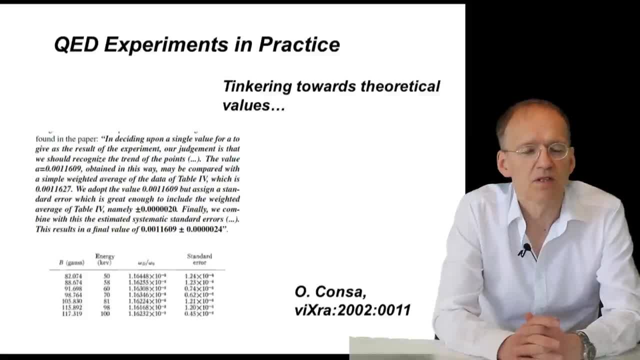 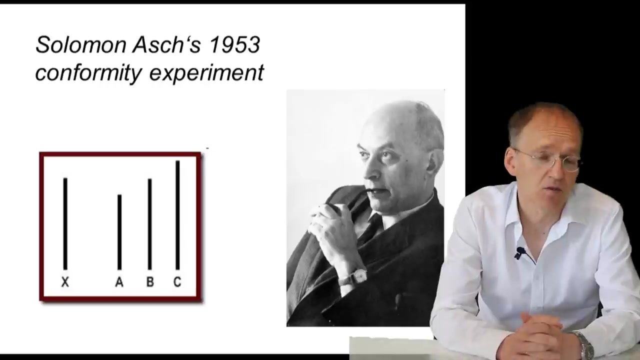 Because if you are a researcher rooted in your community, it is very hard to disagree with hundreds of your skilled and respected colleagues. People judge against their direct perception, as the psychologist Solomon Arsch demonstrated in 1953 in his famous experiment, and the social pressure is much worse here. 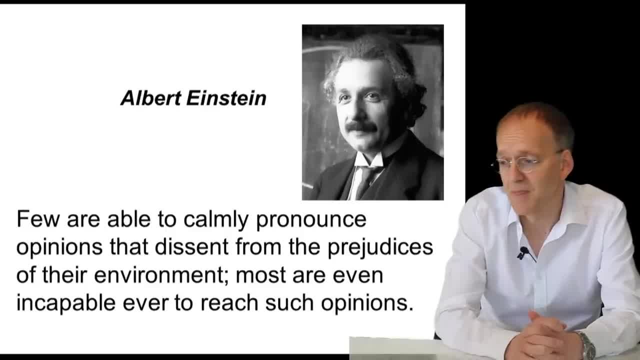 And to remind the quote from Albert Einstein, few are able to calmly pronounce opinions that dissent from the prejudices of their environment. Most are even incapable ever to reach such opinions. And there is another confession I'd like to make. I always liked a lot Richard Feynman. 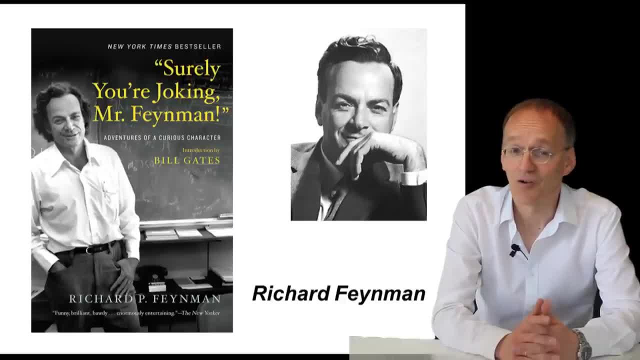 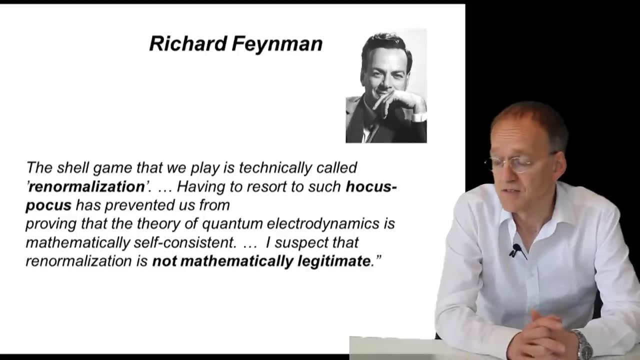 His writings, his frankness, his openness, his mockery of string theory. I just couldn't imagine that his theory, his Nobel, was just a bunch of nonsense. But he even knew it. he admitted it, Aware of Dyson's destruction. he said: 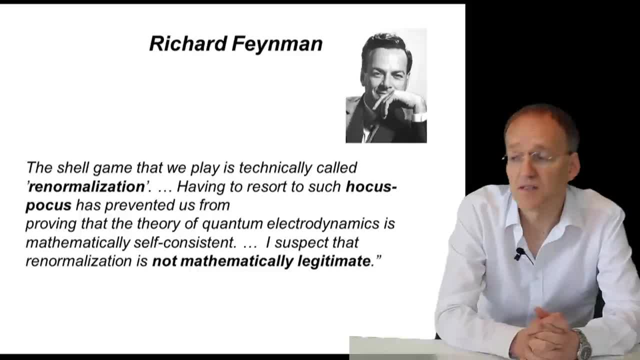 the shell game that we play is technically called renormalization. Having to resort to such hocus-pocus has prevented us from proving that the theory of quantum electrodynamics is mathematically self-consistent. I suspect that renormalization is not mathematically legitimate. 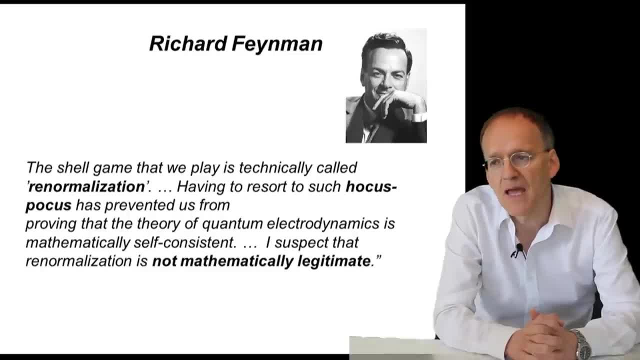 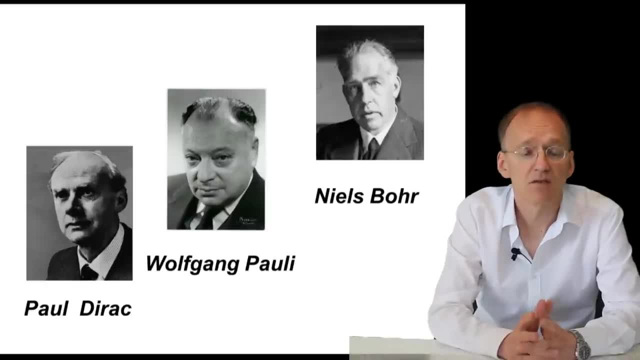 Yet Feynman was too superficial In his reasoning And his biggest blunder was to be dismissive about history. Because they knew it. Dirac knew it wouldn't work. Pauli said it in his Nobel lecture that you could not use renormalization. 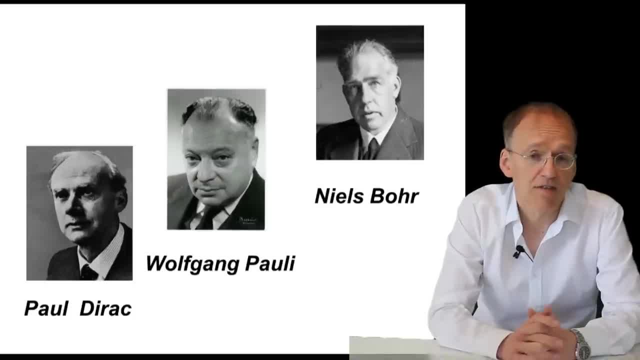 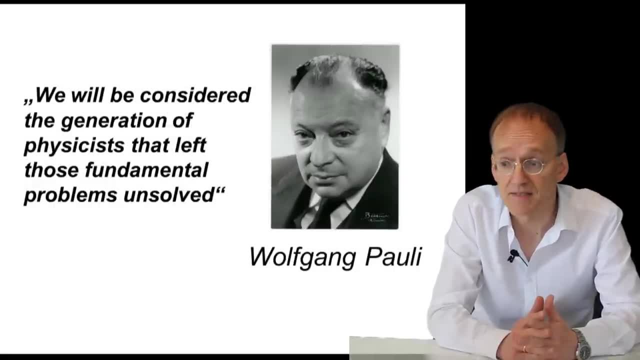 About the unsolved problem of the electron's self-energy. he said we will be considered the generation of physicists that left those fundamental problems unsolved. And Bohr and Schrödinger and Einstein probably did not comment about the idea of renormalization. 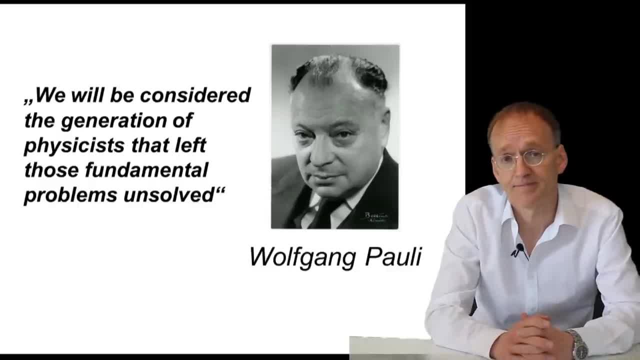 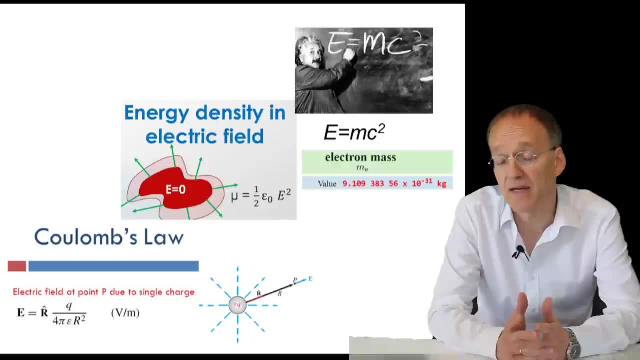 because they considered it an approach too dumb to mention. Indeed, it is as simple as this. There are three formulas of established classical physics that, applied to the electron, contradict each other. There is Coulomb's law of electrodynamics. there is the energy density of the electric field. 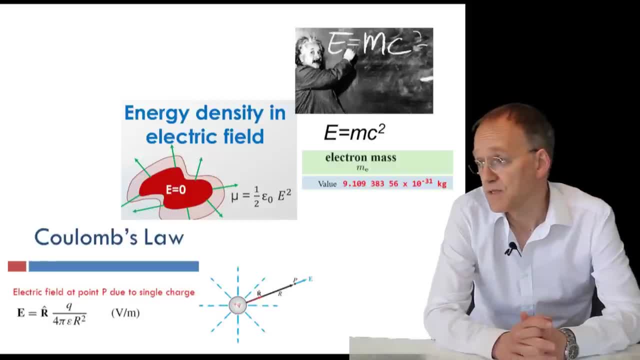 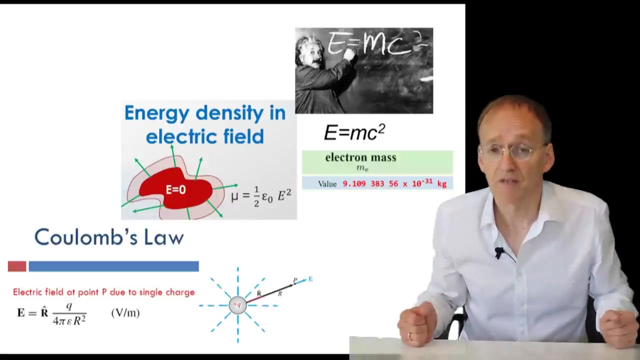 and Einstein's famous E equals mc squared, which links the energy to the mass of the electron. But now, if you apply this and compute the electron's mass, you get an infinite value. So renormalization claims that from this infinite value you can subtract a so-called naked mass of the electron. 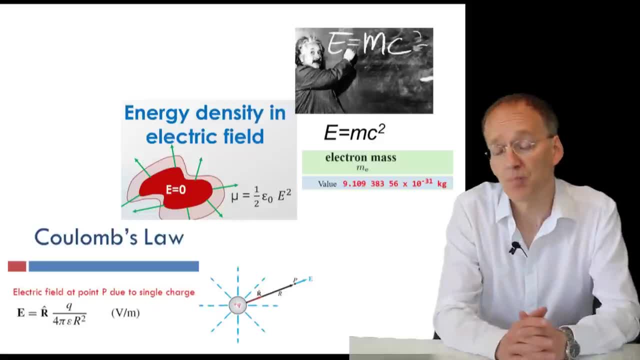 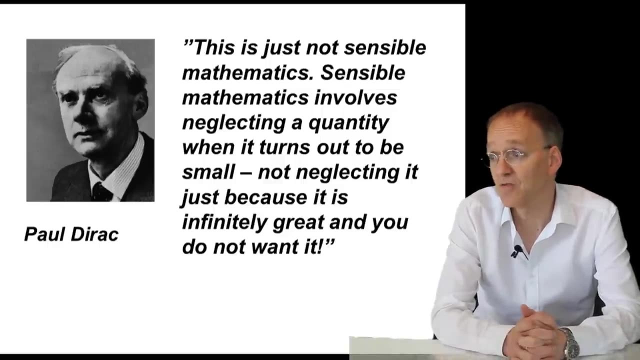 whatever that means, and you get, voila, 9.11 x 10 to the minus 31. kilograms. that's nonsense. and Dirac commented: and there's nothing to add. this is just not sensible mathematics. sensible mathematics involves neglecting a quantity when it turns out to be small, not neglecting it just because it's. 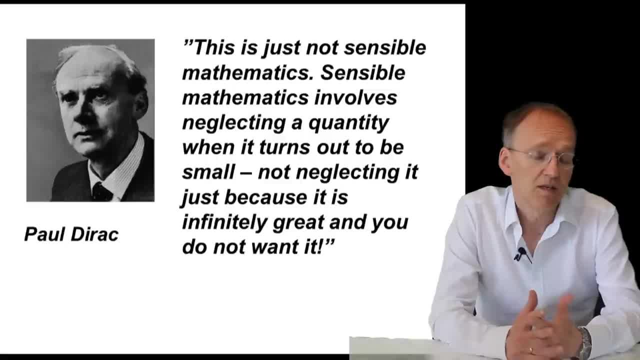 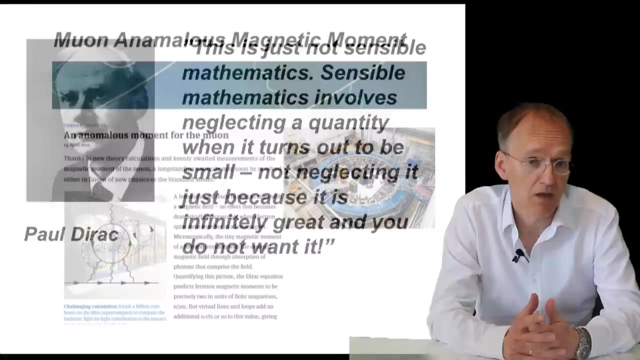 infinitely great and you don't want it. so QED was a stillborn baby from the outset and, yes, what happened in the last 70 years is collective insanity. but to be realistic, it is very hard to admit for any scientist professionally involved in QED. so with this new muon anomaly contradicting QED, it has 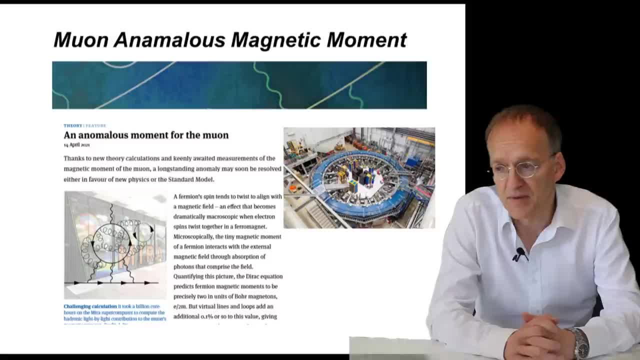 fallen flat on its nose again. but over the course of 70 years the theory has developed a theory that says that QED is not a natural phenomenon, but rather a theory that says that QED is not a natural phenomenon, but rather a such an unhealthy elasticity that it can accommodate any experimental 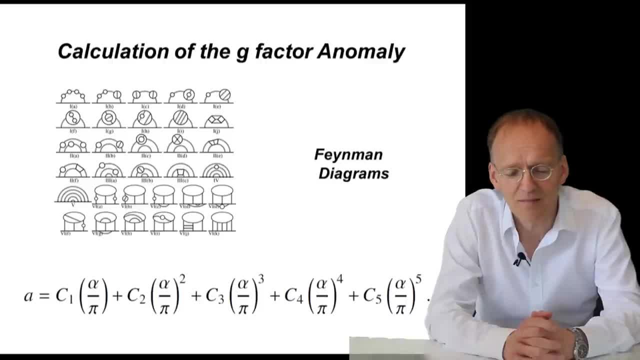 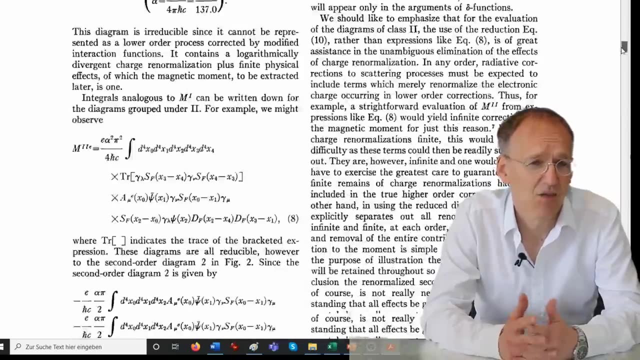 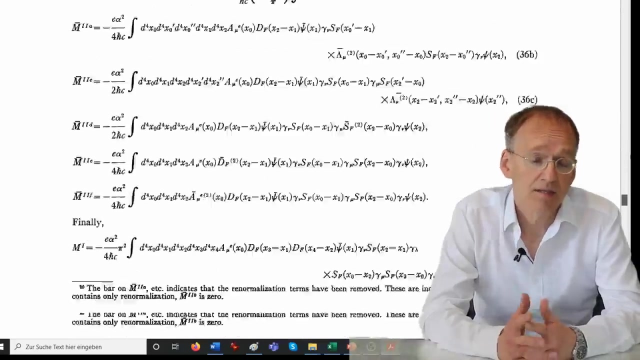 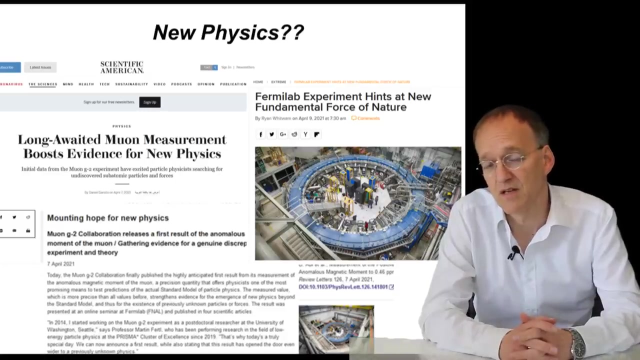 disagreement by construction. a sum to which you can add arbitrary terms with ill-defined factors that does not even converge, can be equated to any number. they have opened the floodgates to a non falsifiable, non science which has reached the state beyond hopeless. this is hard to digest and this is why the new results are interpreted in the 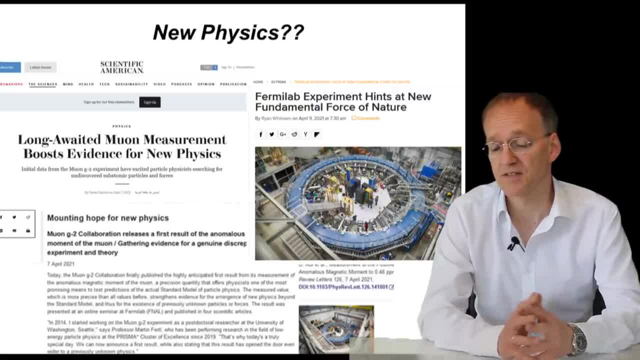 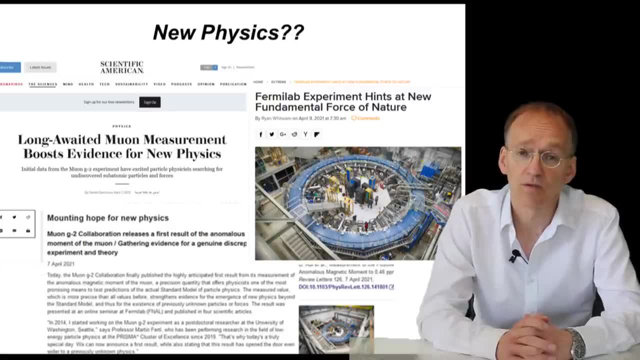 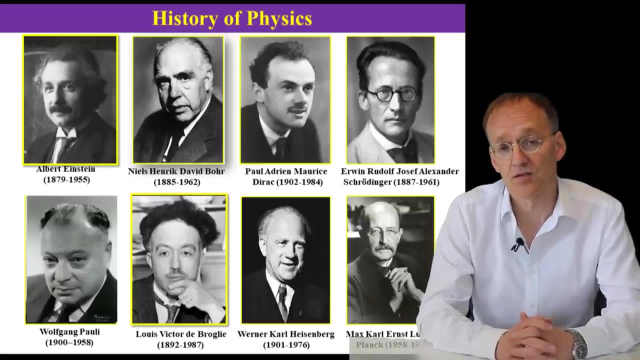 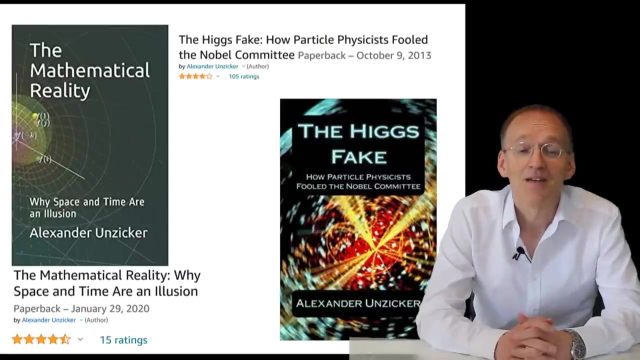 anomaly is pointing towards new physics or other nonsense. it's a sad story of human self-deception, and if you want to understand fundamental physics, you have to go back at least to 1930 and start over. and since this channel is about fundamental physics, this had to be said. if you enjoyed the video, don't. 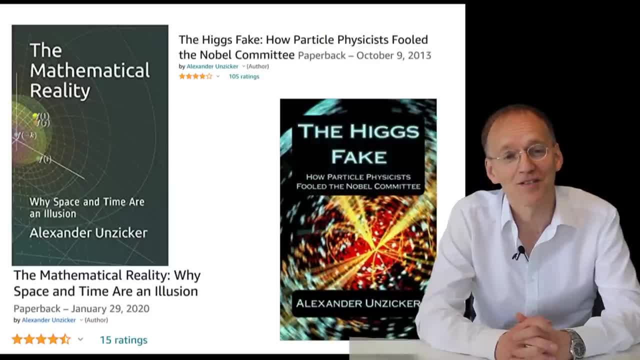 forget to like it and if you're interested in fundamental physics, subscribe to this channel.